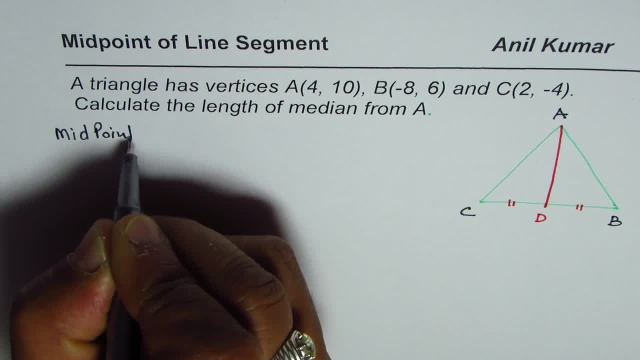 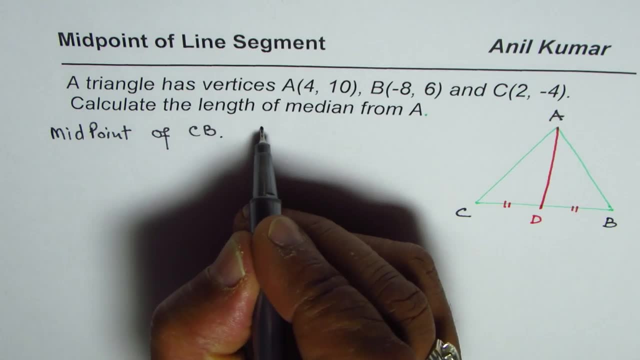 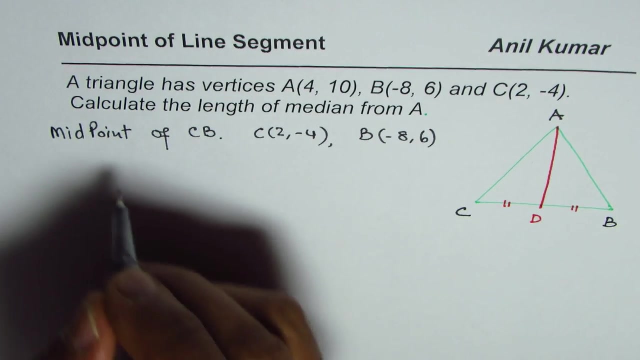 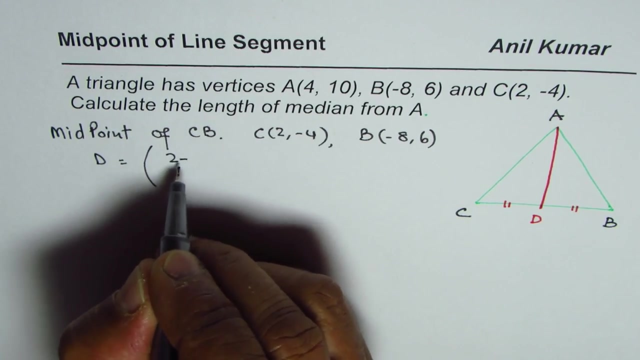 Midpoint of CB right Coordinates of C are 2, minus 4, and that of B minus 8, 6. So the coordinates of point D will be average of these two, So we will add them up. So plus minus 8 means minus 8 divided by 2, and the y value will 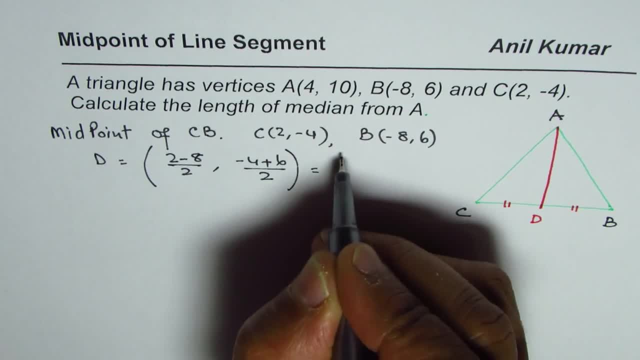 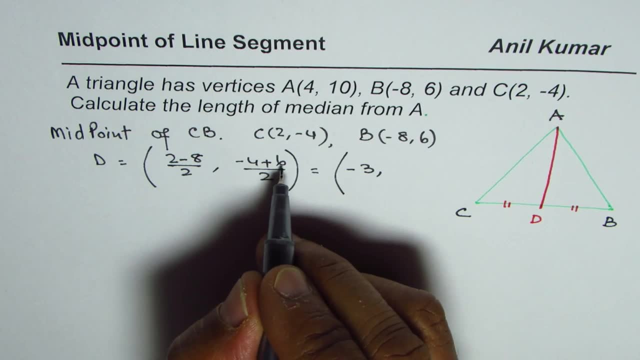 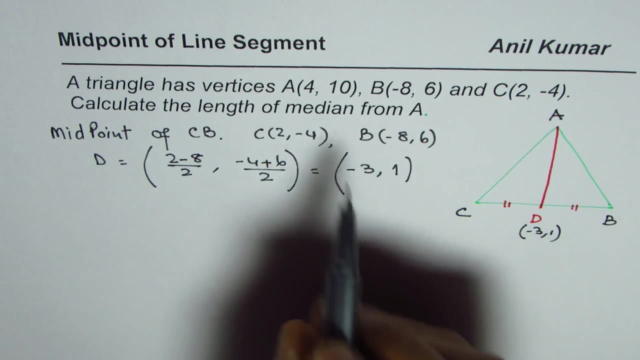 be minus 4 plus 6 divided by 2.. And that is 2 minus 8 is minus 6, divided by 2 is minus 3, and minus 4 plus 6 is 2.. 2 divided by 2 is 1.. So the coordinates of point D are minus 3, 1.. We are given coordinates of 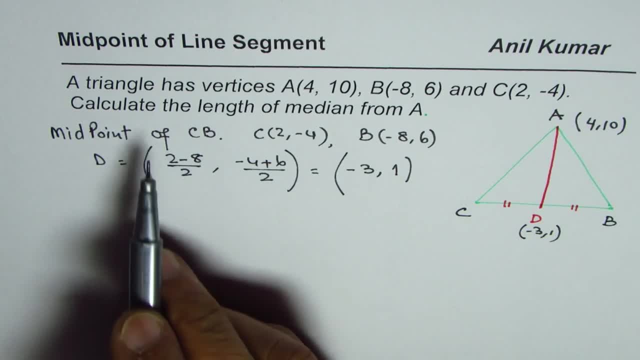 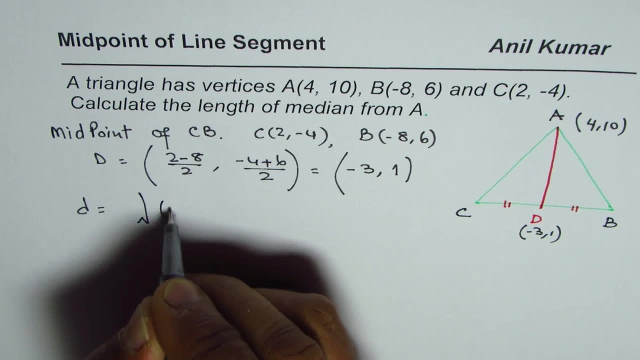 point A, which are 4, 10.. Now to calculate the median we will apply the formula That is: distance D is equals to square root of x2 minus x1, whole square, plus y2 minus y1 whole square. 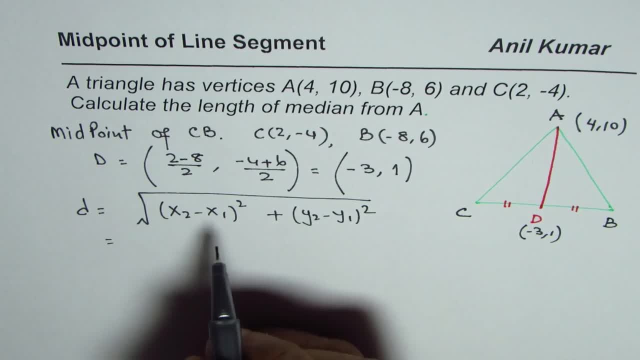 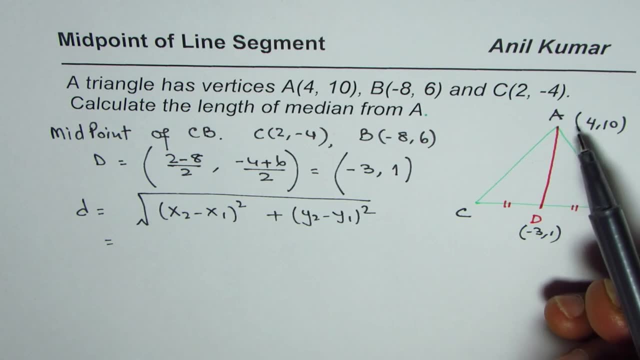 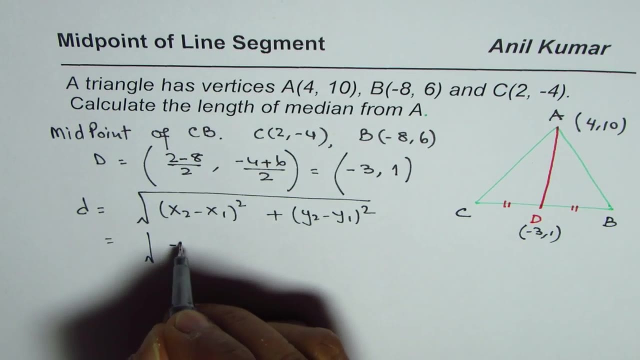 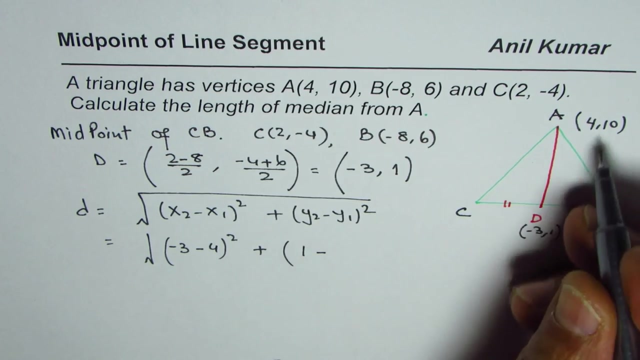 right. So that is the formula Now here we know x1 and x2, these are the values x1 and x2, we can treat x1 as point A, okay, and x2 as minus 3.. So that is minus 3 minus 4 whole square, plus y2: 1 minus 10 whole square square. 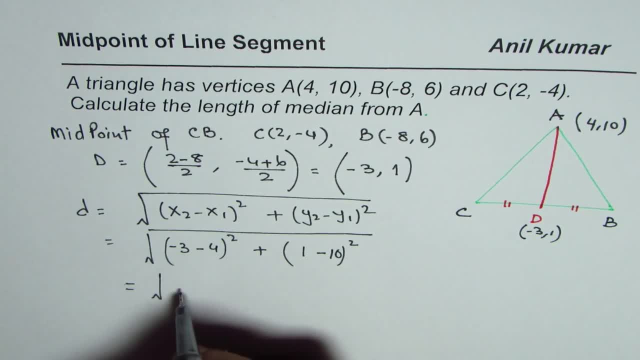 root. So that distance will be: that is 7 square Plus. we can write it in brackets. Since this is negative, let me write negative 9 square. You can use calculator at this stage to answer the question. So we have square root of 7. 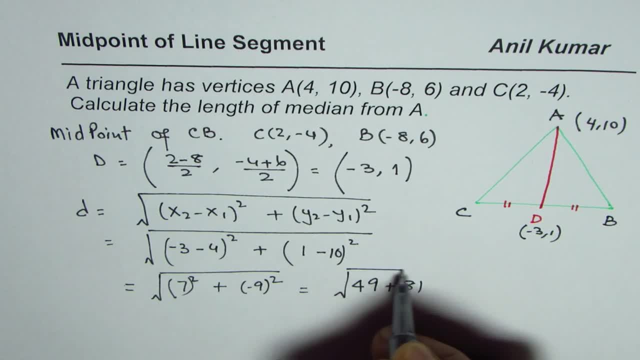 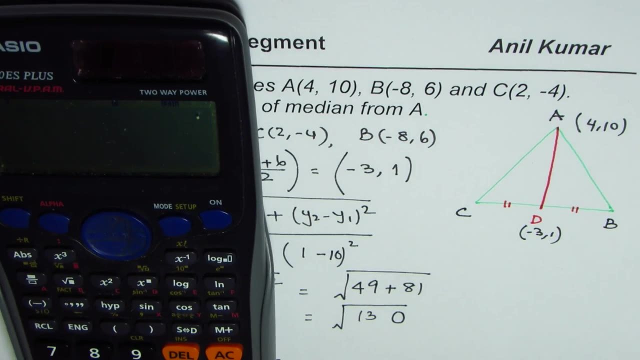 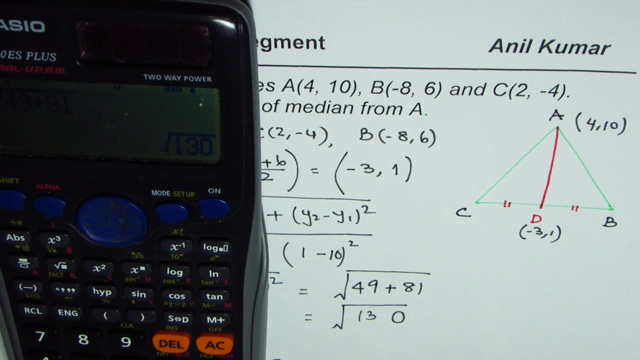 square is 49 plus 9 square is 81. It has to be positive. So when you add them up you get 0 and 130 square root, which you can calculate using the calculator. Square root of- let me write: 49 plus 81 equals to square root of 130, which is equal to.